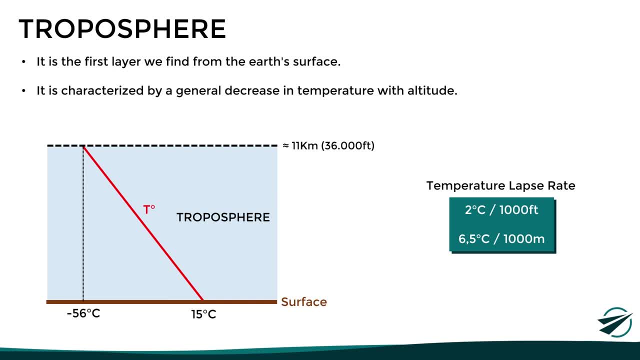 since in reality the temperature in the troposphere can sometimes remain constant with altitude, or even increase slightly when there is an inversion. but that will be discussed in another video. Now you might be wondering: why does the temperature have this tendency to decrease? 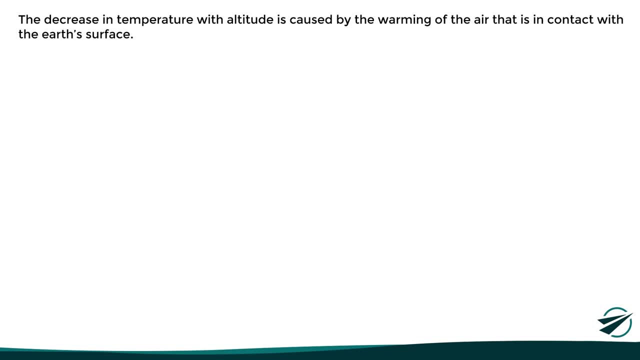 in the troposphere. Well, in this layer, the decrease in temperature will be the same as the decrease in temperature in the troposphere. The decrease in temperature with altitude is caused by the warming of the air that is in contact with the earth's surface. For example, during the day, the surface heats up due to solar 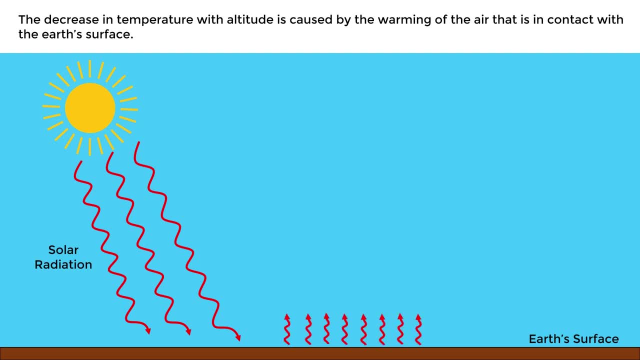 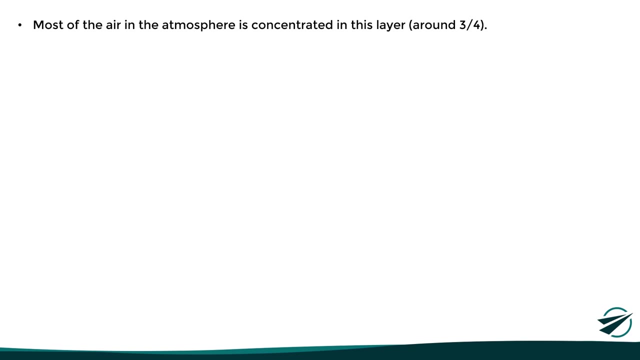 radiation and in turn, this hot surface heats the air that is directly in contact with it. This results in higher temperatures near the surface and colder temperatures at higher levels. Another characteristic of the troposphere is that most of the air of the entire atmosphere 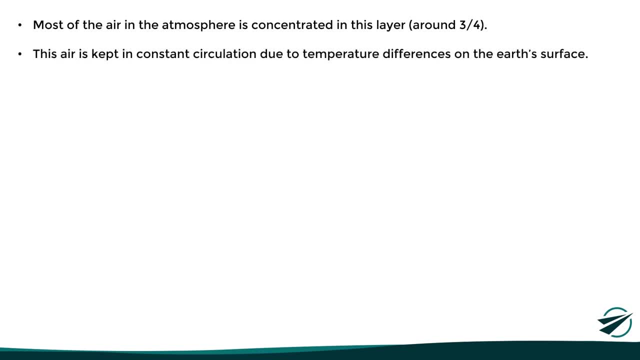 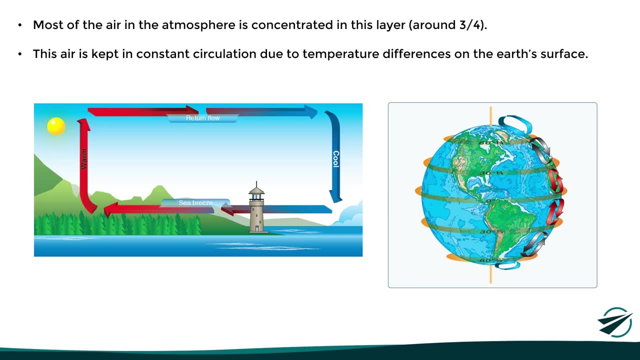 is concentrated in this layer And this air, as you can see, is concentrated in this layer And this air is kept in constant circulation due to temperature differences on the earth's surface, generating wind and convective currents. So, in general, we can say that the air tends to be. 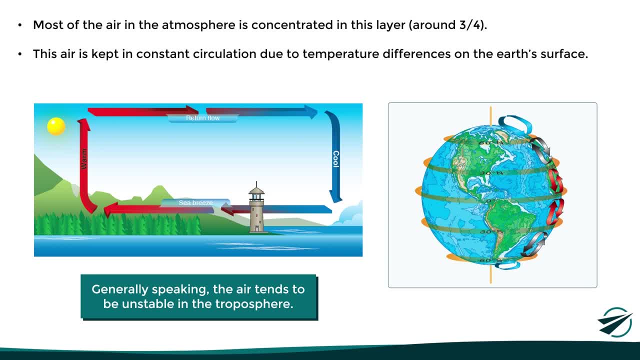 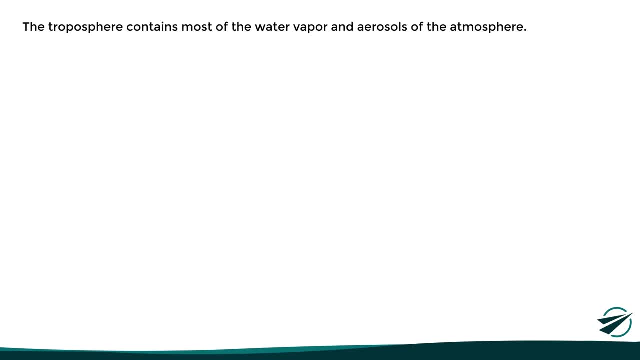 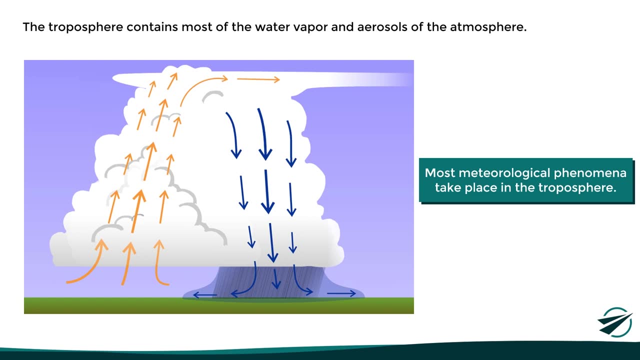 unstable in this layer. Now, another important thing with respect to the troposphere is that it also contains most of the water vapor and aerosols of the atmosphere. This, combined with the fact that the air here is unstable and constantly circulating, implies that most meteorological phenomena, such as the atmosphere- such as the atmosphere and the atmosphere- can also be affected by this layer. 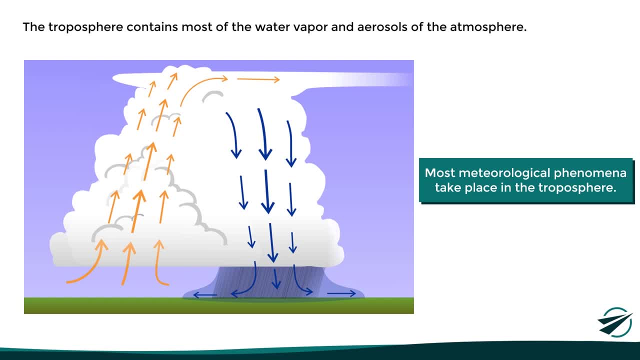 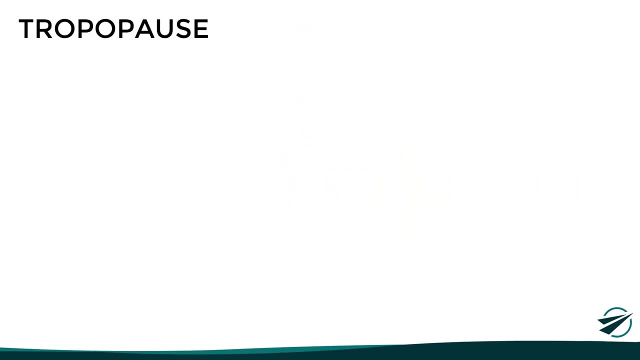 such as thunderstorms and precipitation, take place in this layer. So, having already seen the troposphere, let's move on to the first transition layer, which is the tropopause. This is a thin layer that marks the boundary between the troposphere and the stratosphere. 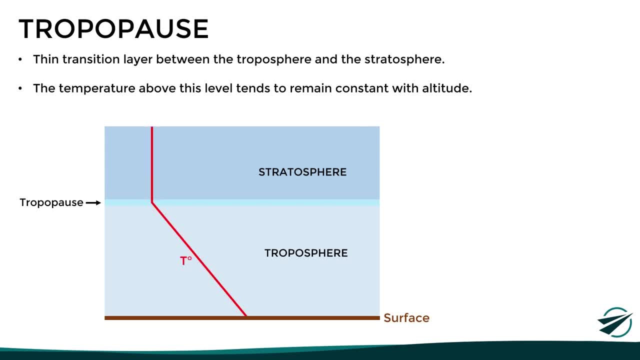 Its main characteristic is that the temperature lapse rate changes abruptly and it now tends to remain constant with altitude. Now, as we said previously, the average upper limit of the troposphere is around 11 kilometers or 36,000 feet. However, since, in reality, the extension of the troposphere varies, this means that the 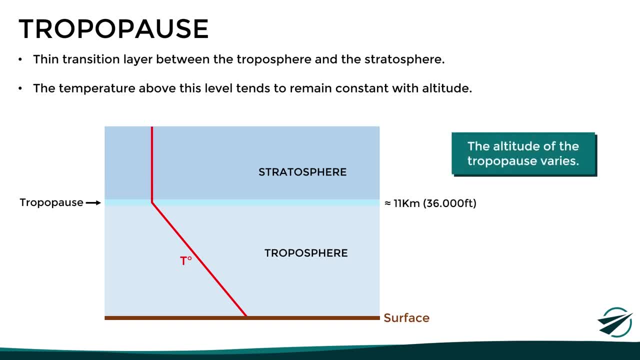 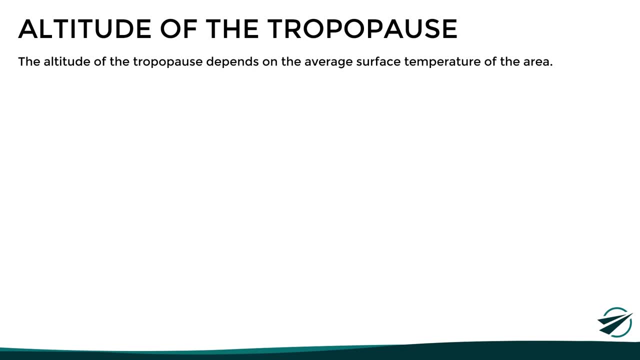 altitude of the tropopause also varies. In fact, the altitude of the tropopause depends mainly on the average surface temperature of the area. This way, if there is a low surface temperature, the air above it will tend to shrink and therefore we will have a lower tropopause. 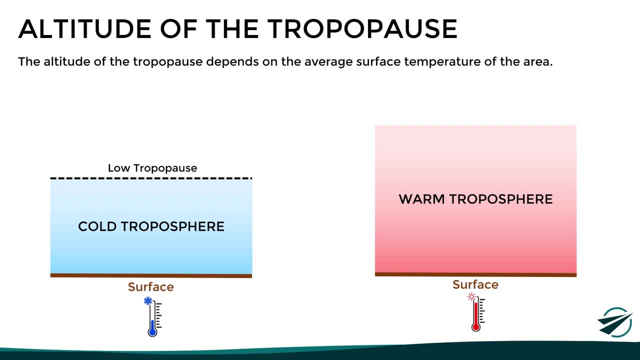 On the other hand, if there is a high surface temperature, the air above it will tend to expand and therefore we will have a much higher tropopause. With this in mind, it is logical to think that near the equator, where the surface temperature 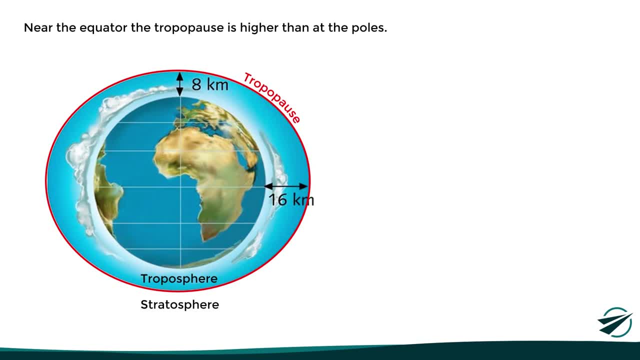 is high, we will have a much higher tropopause than at the poles, where the surface temperature is much lower. Now, although in general terms this is true, the altitude of the tropopause also depends on the seasons and certain climatic phenomena present in a region. 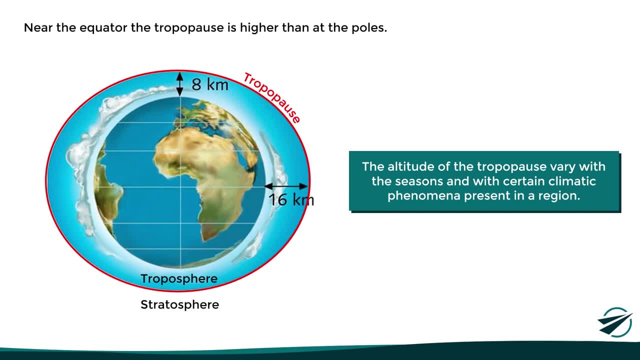 This means that the altitude of the tropopause also depends on the seasons and certain climatic phenomena present in a region, especially in mid-latitudes. But let's go back to the main characteristic of this layer, and it is that the temperature stops decreasing with altitude. 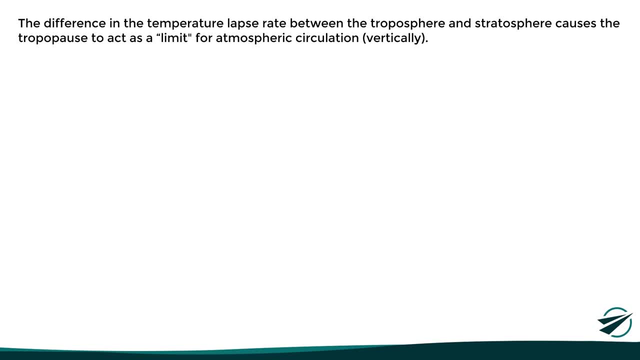 This difference in the temperature lapse rate between the troposphere and stratosphere causes the tropopause to act as a limit for vertical atmospheric circulation. This happens because, as we said earlier, the air in the troposphere is unstable and tends to move both horizontally and vertically. 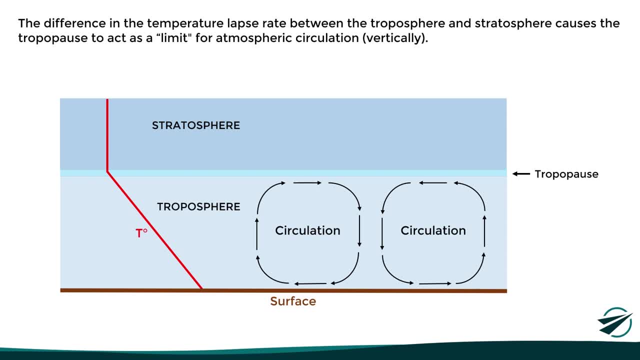 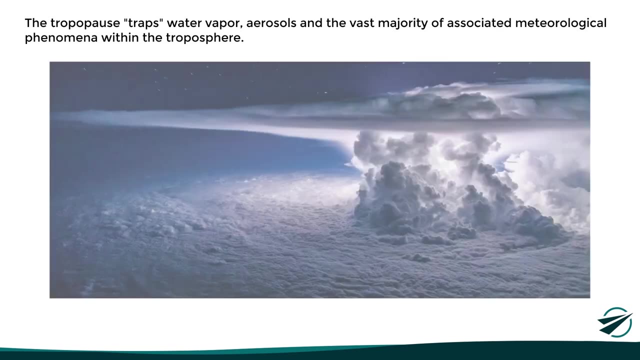 However, if the air reaches the tropopause and the temperature stops decreasing, it becomes more stable, restricting the vertical movements and tending to flow horizontally. only In simpler words, we could say that the tropopause acts as a kind of cap that traps water vapor. 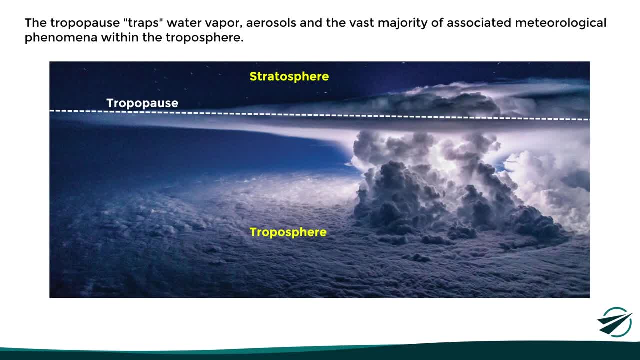 aerosols and the vast majority of associated meteorological phenomena within the troposphere, preventing them from extending up to the stratosphere. A clear example of this is the vertical development of some climatic phenomena. A clear example of this is the vertical development of some climatic phenomena. 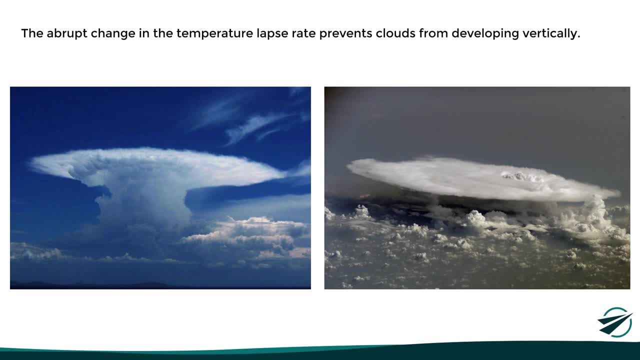 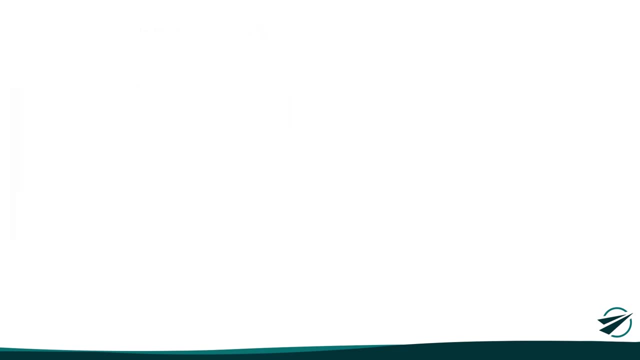 In these images, we can see how the abrupt change in the temperature lapse rate of the tropopause prevents these clouds from continuing to develop vertically into the stratosphere. Now, taking into account all that we have seen so far, we could think that the altitude 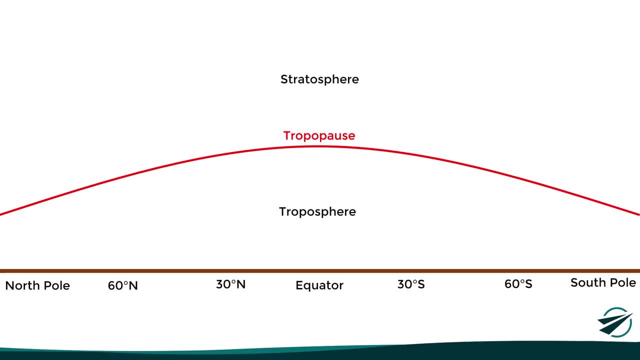 of the tropopause changes gradually and continuously between the equator and the poles, as shown here. However, in reality, things are a little different. Since the distribution of atmospheric sunlight and the temperature of the tropopause changes, the altitude of the tropopause increases automatically. 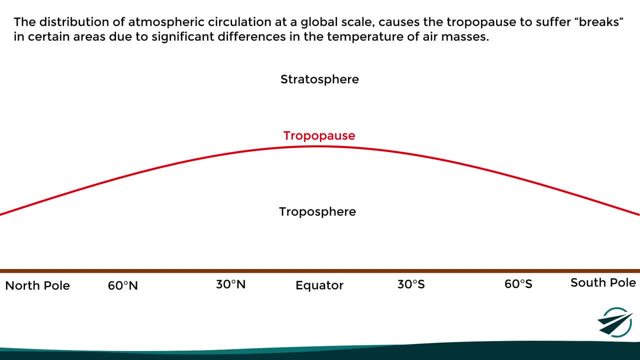 As shown here, circulation at a global scale causes the tropopause to suffer breaks in certain areas due to significant differences in the temperature of air masses. This way, we rather get a tropopause like this one. As we can see, atmospheric circulation within the troposphere is divided. 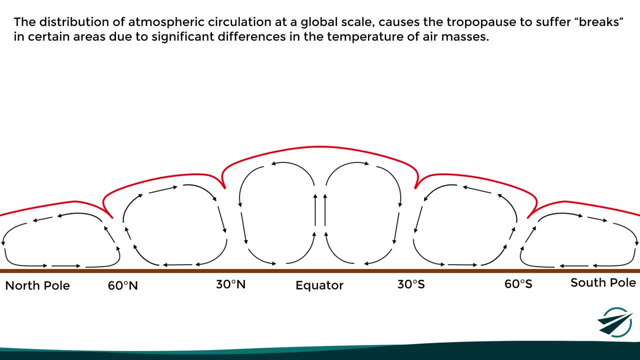 into different cells. The ones closer to the equator are known as the Habli cells, The ones located in mid-latitudes are the ferrocells, and the ones over the poles are called polar cells. With this distribution, instead of having a single tropopause, we end up with individual. 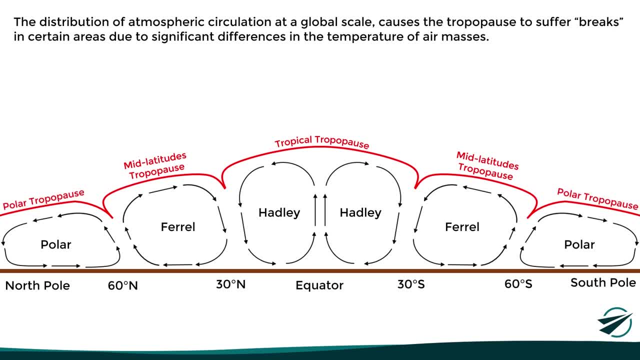 tropical, mid-latitude and polar tropopause. Tropical tropopause is the highest of all, reaching altitudes of around 16 kilometers or 53,000 feet, and temperatures of minus 80 degrees Celsius. Mid-latitudes tropopause is typically found at 11 kilometers or 36,000 feet, with 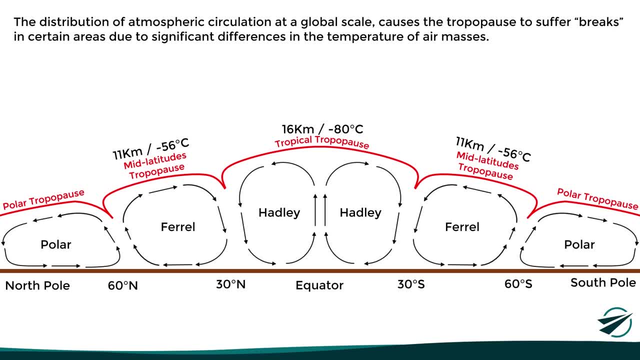 temperatures around minus 56 degrees, but we have to say that it is a tropical tropopause. And finally, polar tropopause is the lowest of all, reaching altitudes of around 8 kilometers or 26,000 feet, and temperatures of minus 40 degrees. Now these breaks in the tropopause. 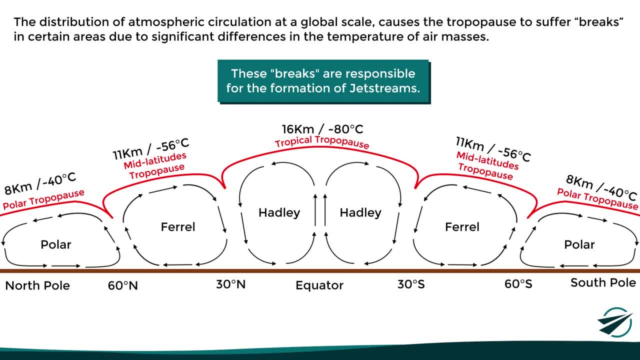 found at approximately 30 and 60 degrees latitude, are also responsible for the formation of jet streams, which are narrow bands of high-speed winds. Specifically, depending on the latitude, we can find the tropopause. in the tropopause, which is the lowest of all reaching altitudes. 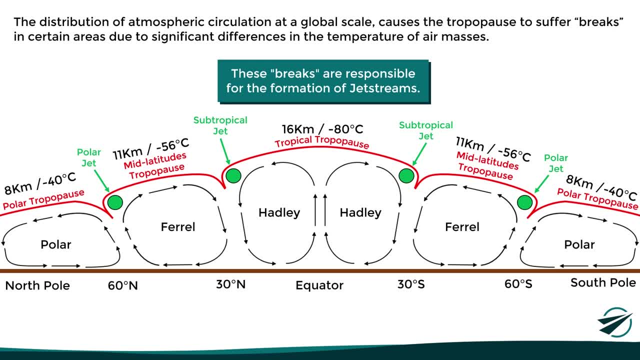 of around 16 kilometers or 36,000 feet and temperatures of minus 40 degrees Celsius, A subtropical or polar jet stream. In this image we cannot appreciate them very well, since we are looking at the atmosphere from the side, but here we can see them better from. 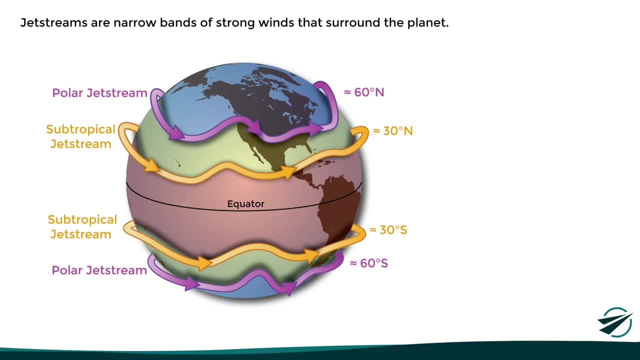 another perspective. The presence of these jet streams greatly influences the performance of aircraft flying close to them, as they can be used to increase ground speed and reduce flight time and fuel consumption or, depending on the situation, they can also be detrimental to flight performance if the aircraft flies against them. 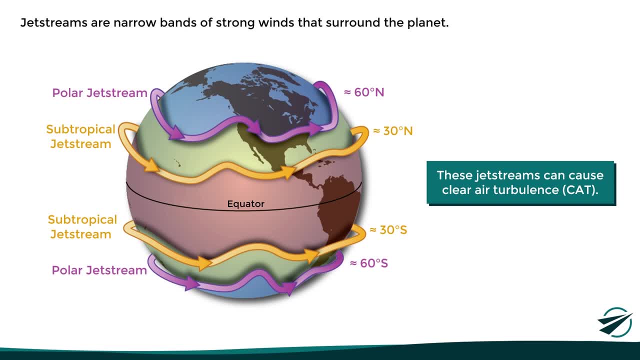 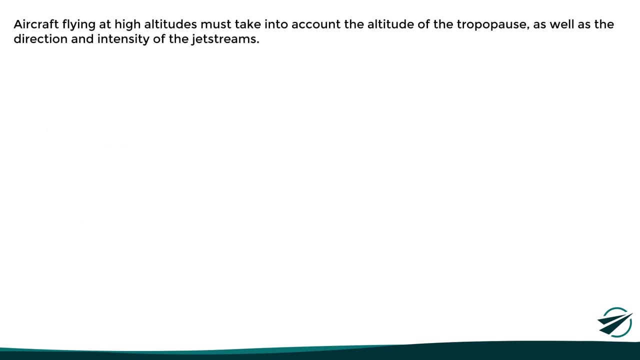 In addition to this, these jet streams can also cause severe, clear air turbulence, which we will discuss in more detail in a future video. Now, since these jet streams are directly related to the altitude of the tropopause, aircraft flying at high altitudes must take into account the altitude of the tropopause. 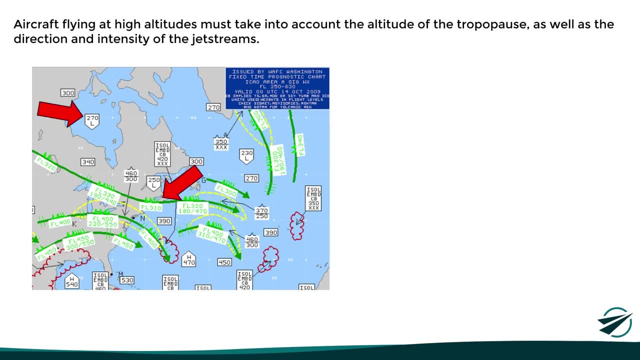 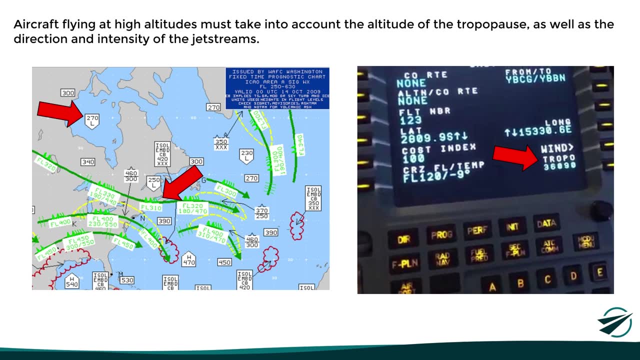 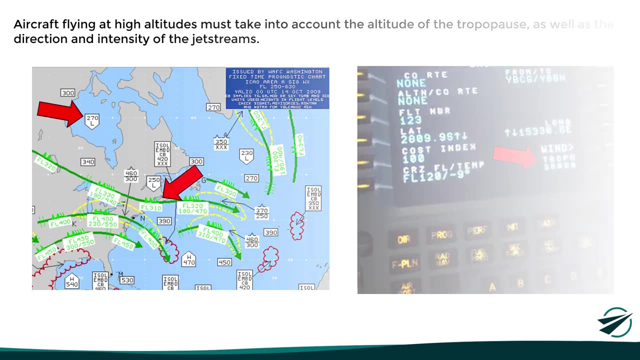 as well as the direction and intensity of the jet streams. In some cases, it is even required to insert this altitude in the flight management systems of some aircraft for more accurate cruise performance calculations. So now that we have seen the most important facts about the tropopause, 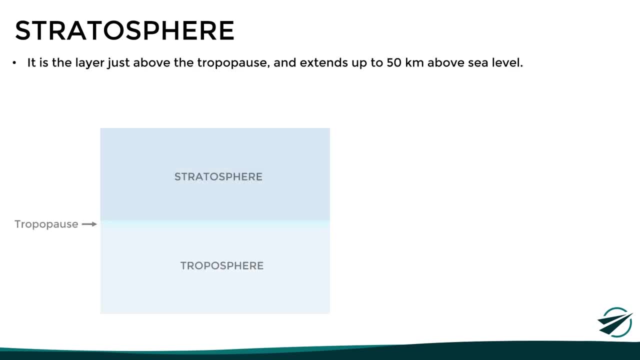 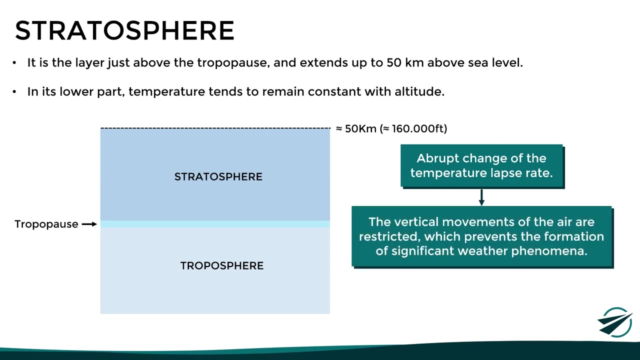 let's move on to the stratosphere. This layer is found just above the tropopause and extends up to an altitude of 50 kilometers or 160,000 feet In its lower levels. temperature tends to remain constant with altitude and, as we said previously, this abrupt change of the temperature lapse rate restricts the vertical. 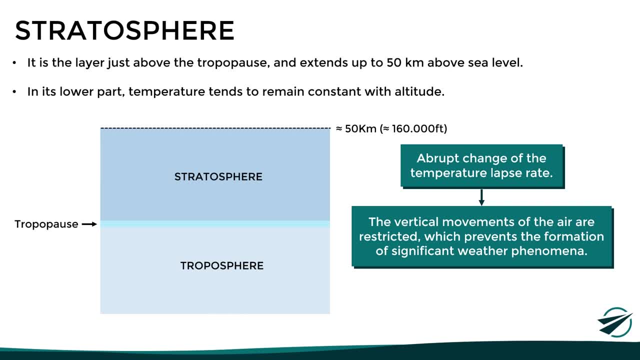 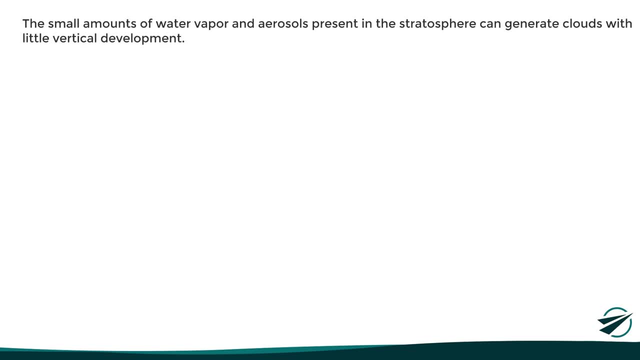 movement of the air, Which, in turn, prevents the formation of significant weather phenomena in this layer. However, we have to say that the small amounts of water vapor and aerosols present in the stratosphere, combined with the low temperatures, can generate clouds with little vertical development. 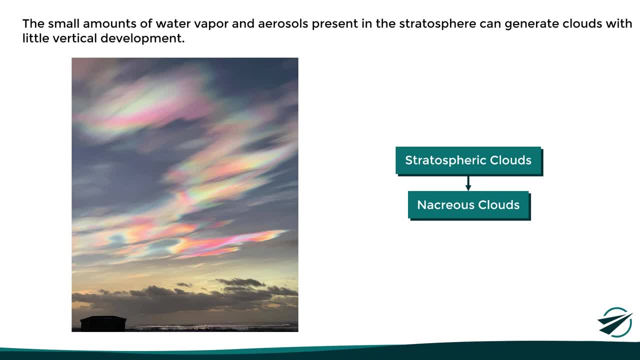 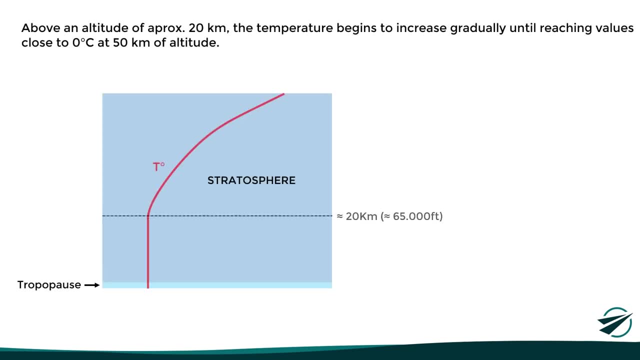 known as stratospheric clouds or nacreous clouds, due to its particular and bright colors. Now, within the stratosphere, above an altitude of approximately 20 kilometers or 65,000 feet, the temperature begins to increase gradually until reaching values close to zero degrees celsius at the top of the stratosphere. 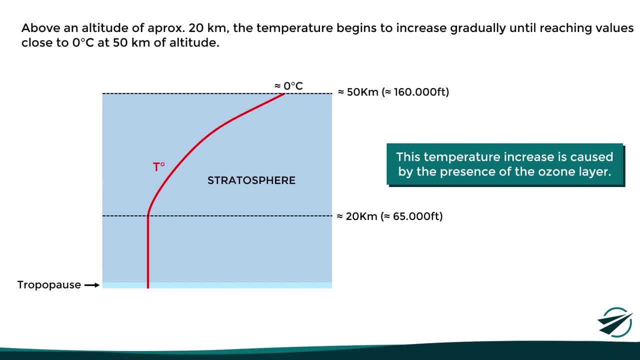 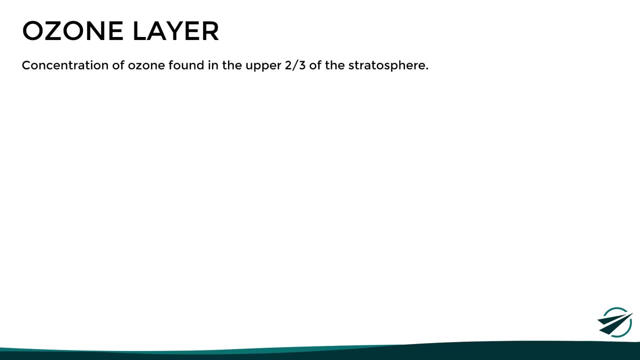 This temperature increase is caused by the presence of the ozone layer. The ozone layer is basically a concentration of ozone found in the upper two-thirds of the stratosphere. But to understand how this influences the behavior of air temperature, we first have to look at what is ozone. 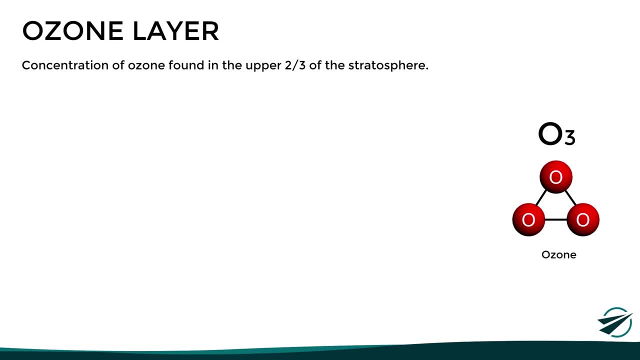 Ozone is a molecule composed of three oxygen, And we have to say that the oxygen in the atmosphere is normally found in the form of molecular oxygen composed of only two oxygen atoms. So what actually happens in this layer is that ultraviolet radiation from the sun breaks the bonds of molecular oxygen. 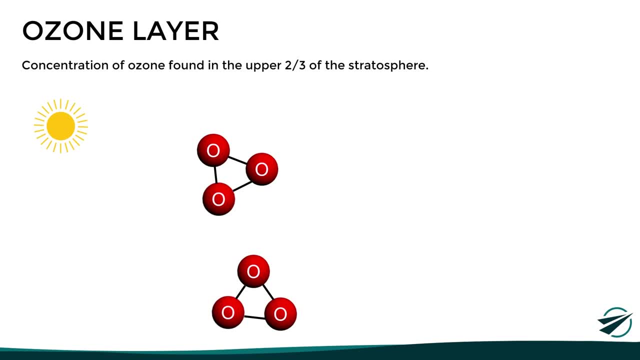 releasing the atoms so that they can bind to other oxygen molecules, thus forming ozone. But the process does not end here. The bonds of this new ozone are broken again by the ultraviolet radiation, Causing the cycle to repeat itself continuously. This continuous process releases heat, which results in an increase in air temperature in this layer of the atmosphere. 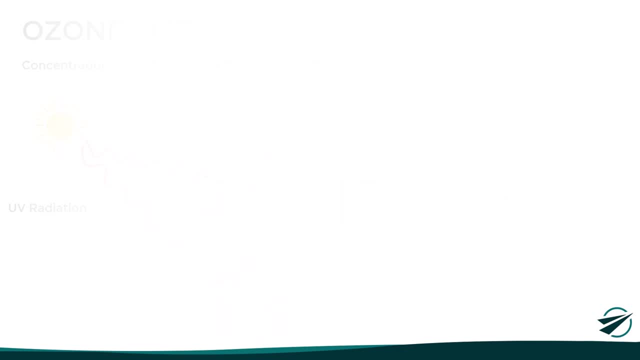 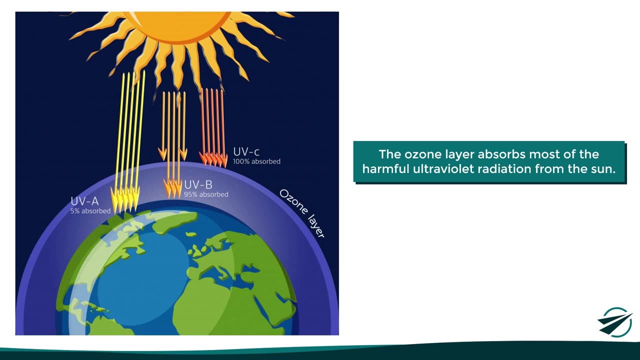 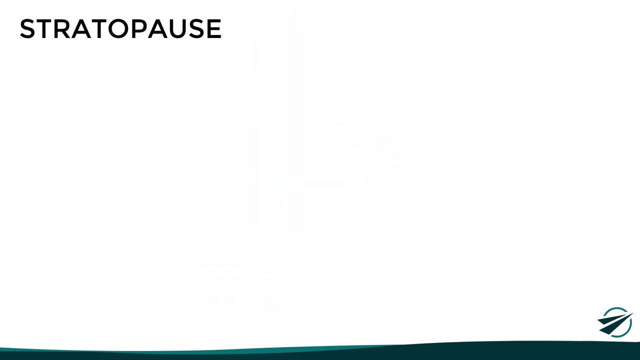 Now, it is also worth mentioning that this ozone layer absorbs much of the more energetic ultraviolet radiation from the sun, which is harmful to most species living on the surface, so it acts as a kind of filter. So, continuing with the layers of the atmosphere, just where the stratosphere ends, we find the stratopods. 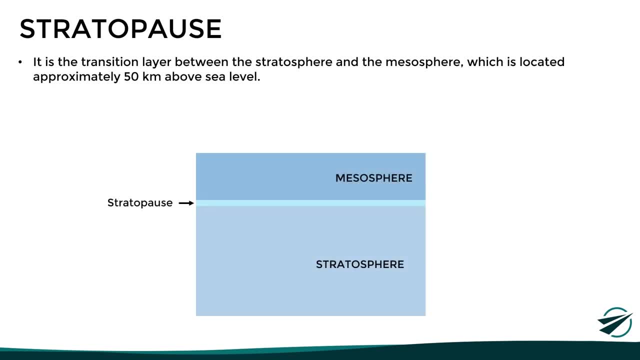 Which is a thin transition layer between the stratosphere and the mesosphere, located at approximately 50 kilometers or 160,000 feet of altitude. Its main characteristic is that, from this level, the temperature stops increasing and tends to remain constant with altitude initially. 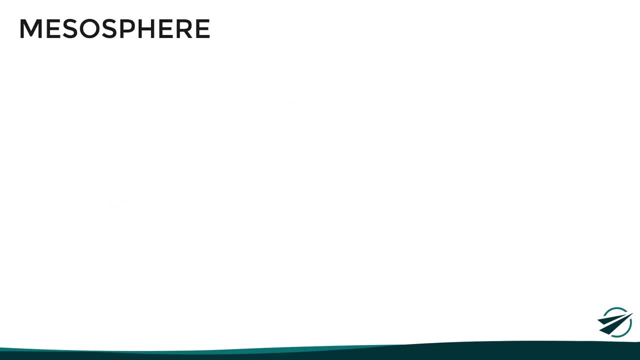 Then, right above this transition layer, we find the mesosphere. This layer extends from the stratopods up to an altitude of around 80 kilometers or 160,000 feet. The main characteristic of the mesosphere is that the air temperature decreases again with altitude. 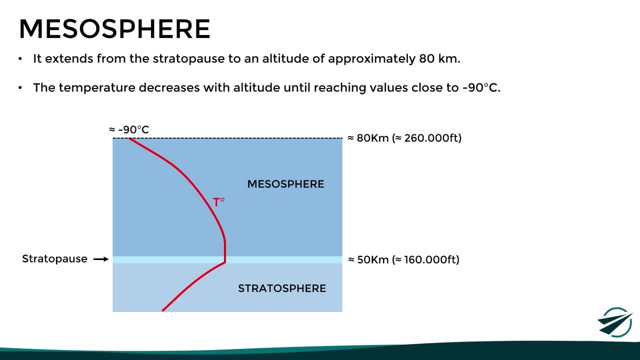 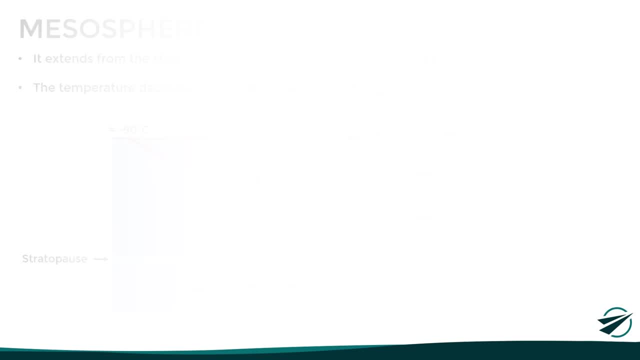 reaching values of around minus 90 degrees at the highest levels, making it the coldest layer of the atmosphere. We should also mention that it is in this layer where most meteorites from space normally disintegrate, which are responsible for meteoro showers and shooting stars. 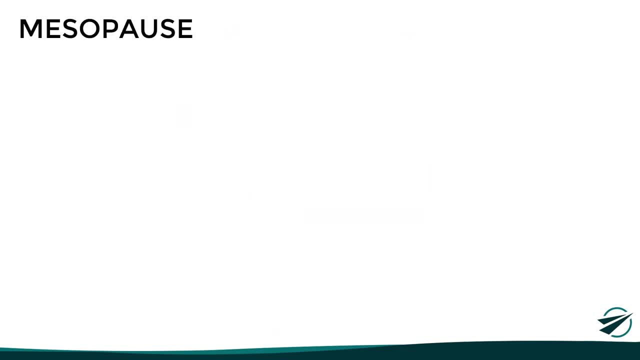 Now, right above the mesosphere, There is the mesosphere mesopause, which is the transition layer between the mesosphere and the thermosphere, and it is found at an altitude of around 80 kilometers or 260,000 feet. Its main characteristic is that temperature stops decreasing and tends to remain constant. 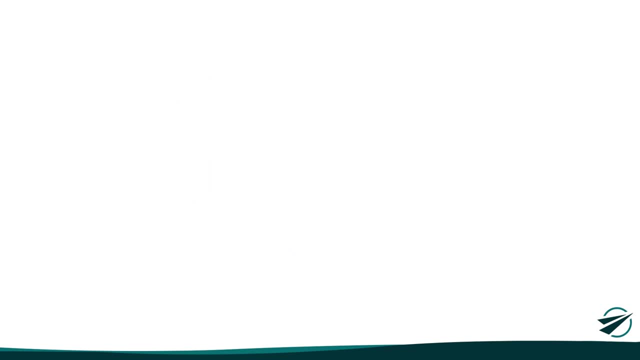 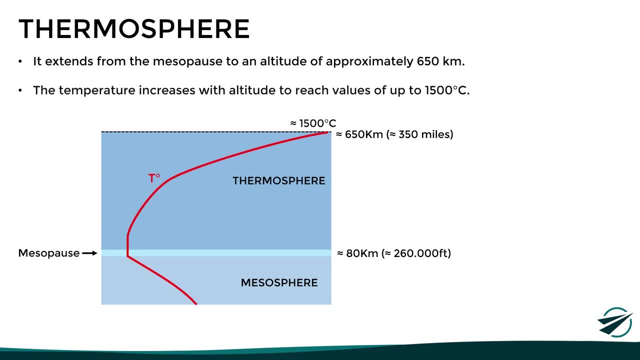 initially, This brings us to the next layer, which is the thermosphere. This layer is pretty thick, since it extends from the mesopause up to an altitude of approximately 650 kilometers or 350 miles, And, as its name suggests, the temperature here increases with altitude reaching values. 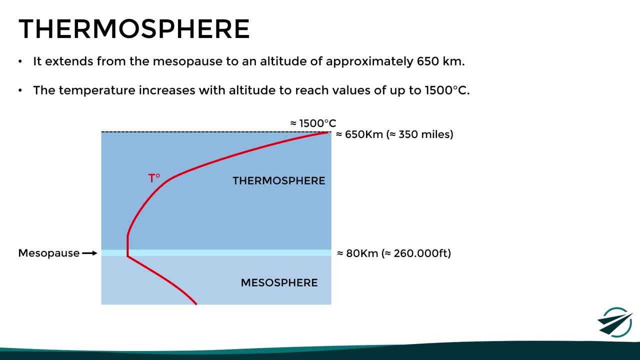 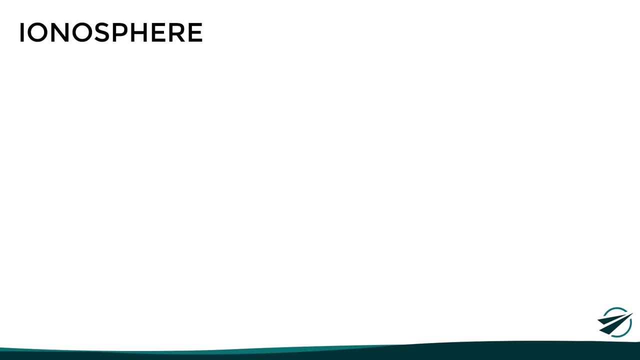 up to 1500 degrees Celsius. However, we must say that the altitude to which the thermosphere extends greatly depends on solar activity, varying between 500 and 1000 kilometers. Now, this significant increase in temperature with altitude is due to the presence of the 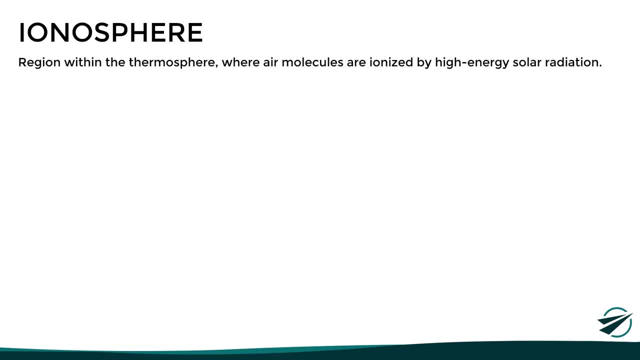 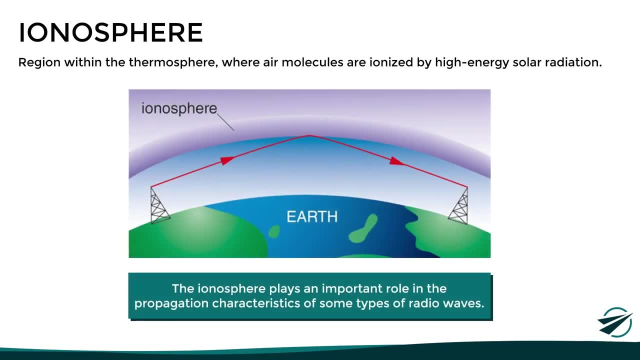 ionosphere, Which is a region within the thermosphere where air molecules are ionized by high-energy solar radiation. This ionosphere also plays a very important role in the propagation of some types of radio waves because, depending on their frequency, some waves pass through it, some are absorbed. 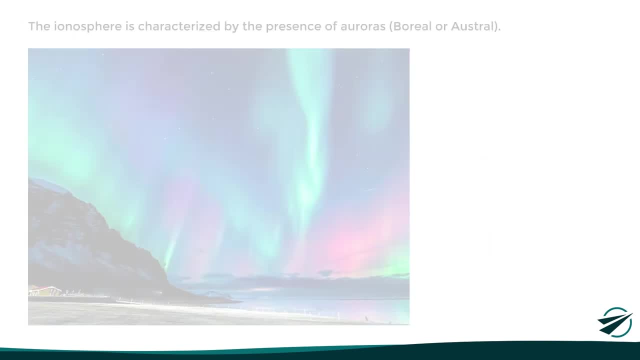 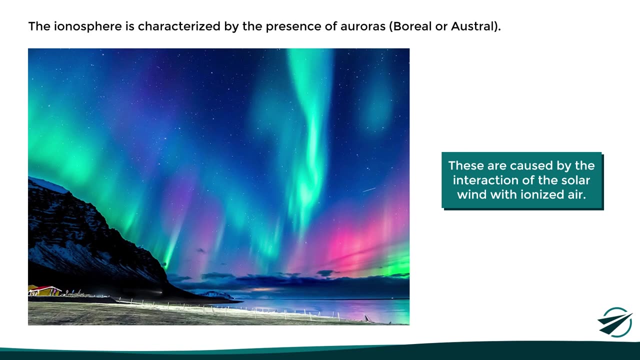 and some bounce back to the surface. Also, this layer is characterized by the presence of auroras in regions close to the poles, which are caused by the interaction of the solar wind with ionized air. This layer is characterized by the presence of auroras in regions close to the poles.